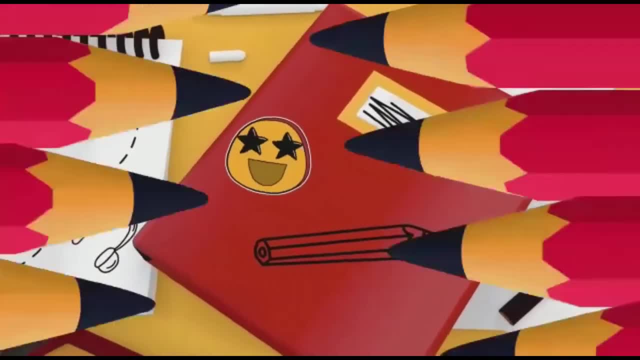 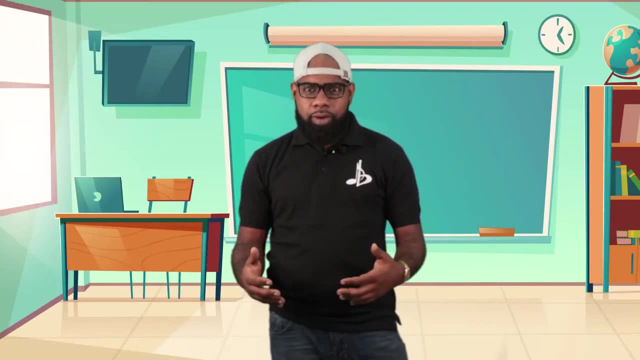 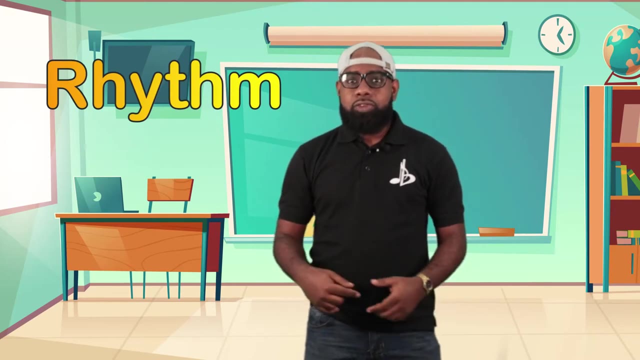 Hey guys, welcome back to the music class. Today we're going to be talking about rhythm. Yep, rhythm. Can you see the word rhythm on the screen? Yes, let's spell that word. Two, three, R-H-Y-T-H-M Rhythm. Good job. 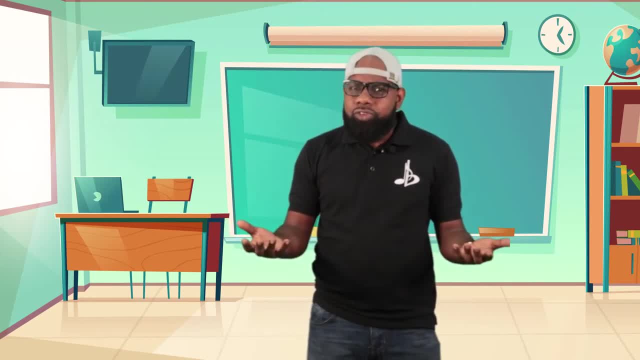 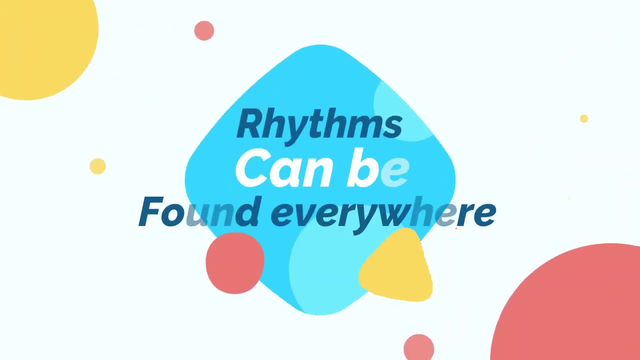 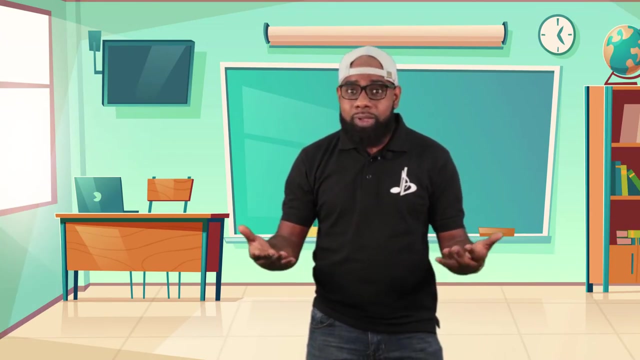 So you might be asking yourself: what is rhythm? I sometimes ask myself that same question and I found the answer. Let's go. So rhythm is a pattern of sound Or words or music. Wait, rhythm is everywhere. Or even dance, Yep, Can you feel that? 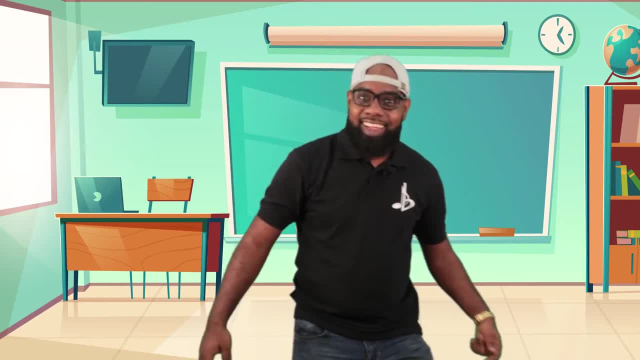 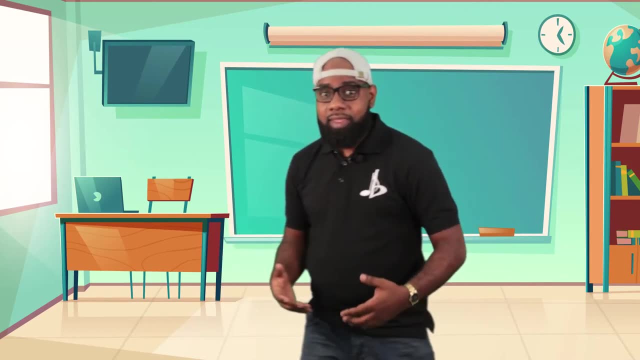 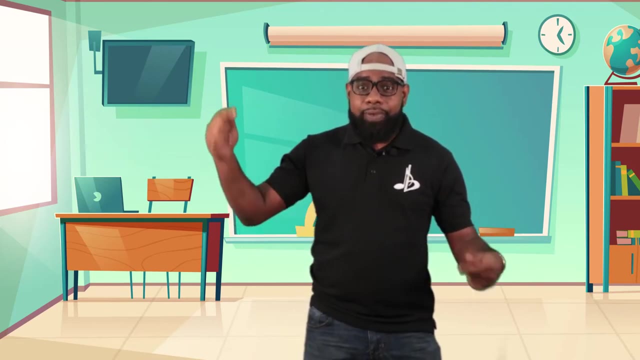 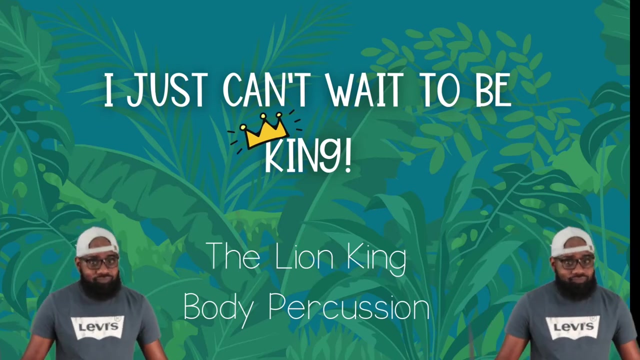 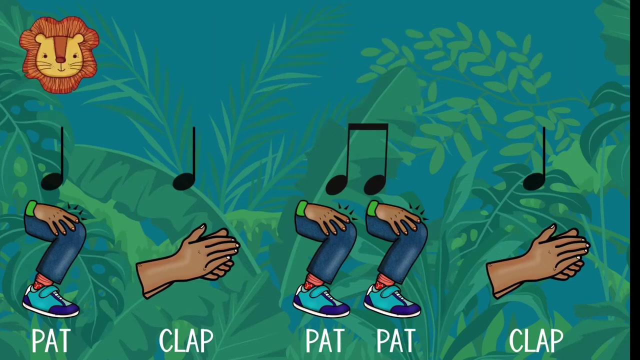 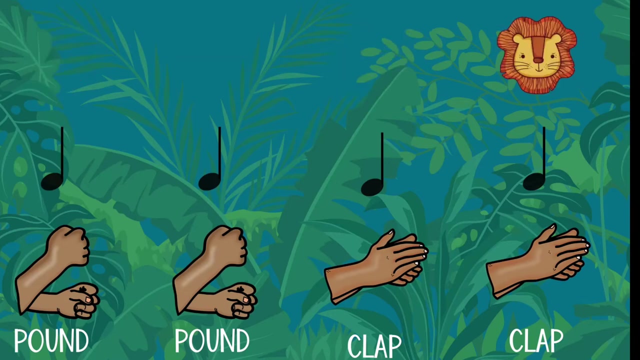 Whoa. Great job, Guys. that was awesome, So it's time to drop that beat. Let's go. I'm going to be a mighty king, so enemies beware. Well, I've never seen a king or beast with quite so little hair. 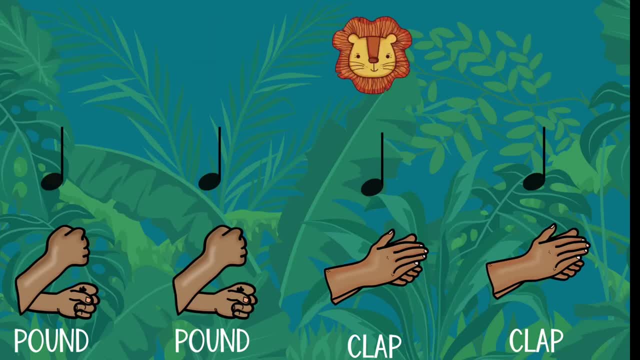 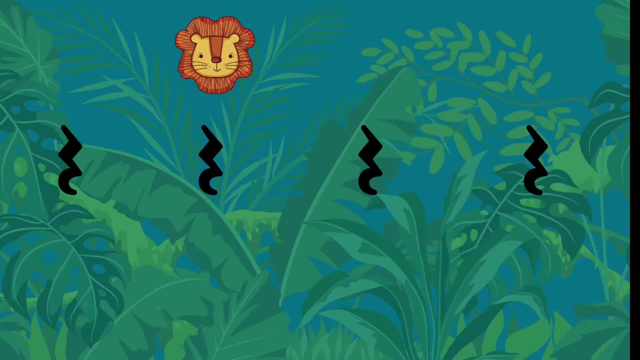 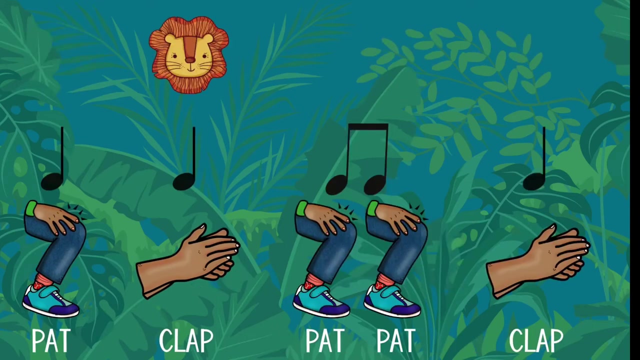 I'm going to be the main event, like no king was before. I'm brushing up, I'm looking down, I'm working on my board This far- a rather uninspiring thing. Oh, I just can't wait to be king. 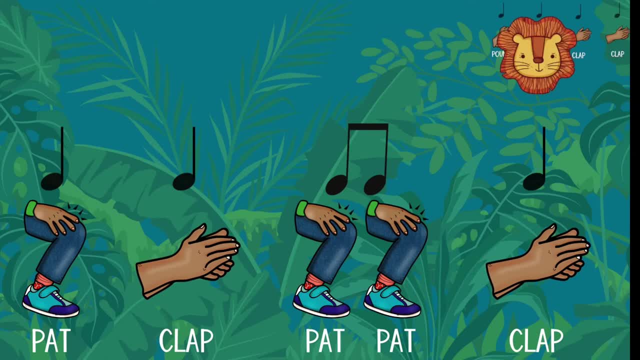 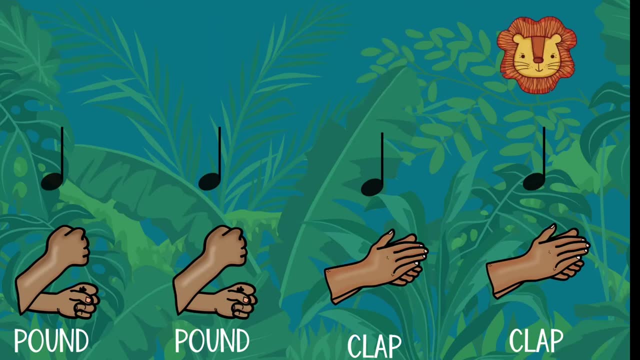 You're off a long way to go, young master. if you think No one's saying, do this. Now. when I said that No one's saying: be there. What No one's saying: stop there. No one's saying: see here. 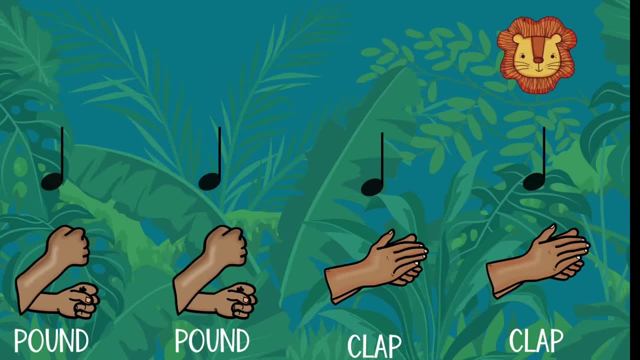 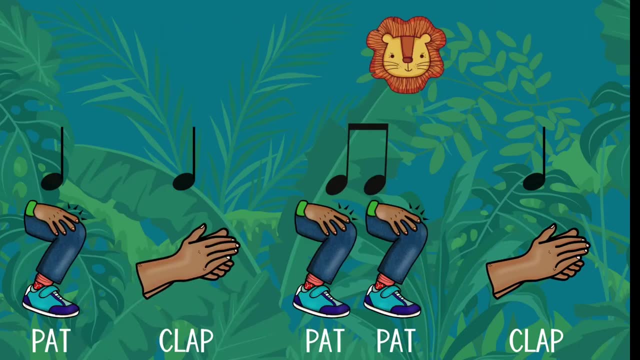 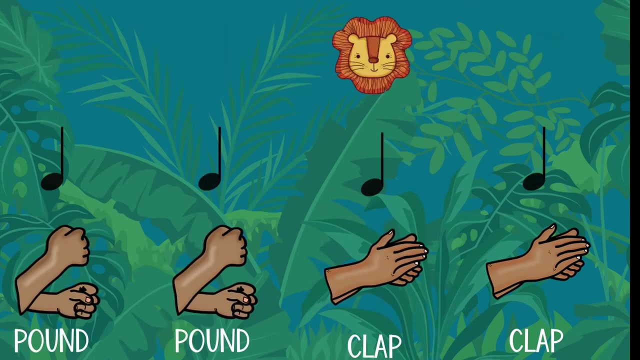 Now see here, We don't run around all day. Well, that's definitely out. We don't do it on my way. I think it's time that you and I arranged a heart-to-heart Kings. don't need advice from little hornbills for a start. 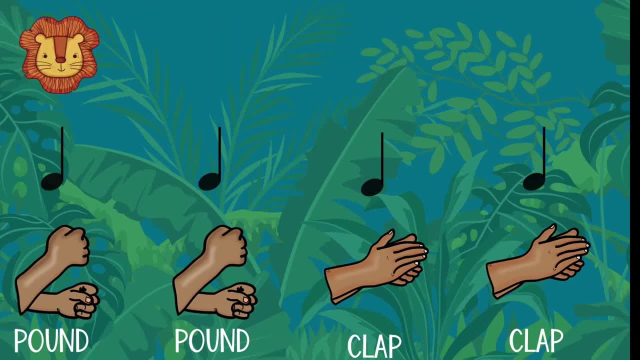 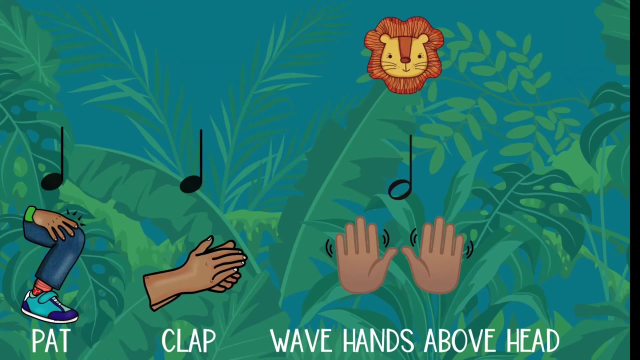 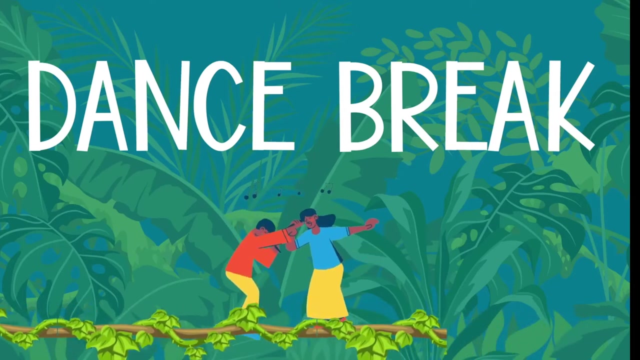 If this is where the monarchy is headed, count me out, Out of service, out of Africa. I wouldn't hang about. This child is getting wild, Wildly out of wing. Oh, I just can't wait to be king. Everybody look left. 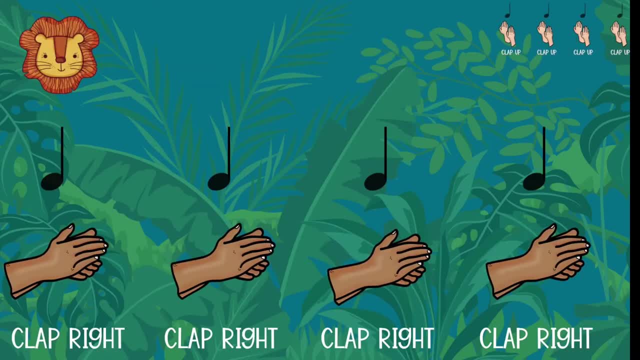 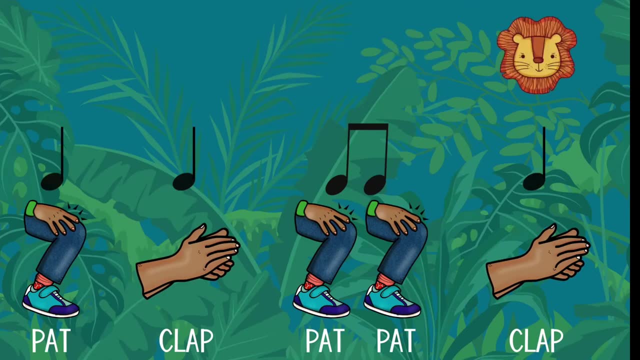 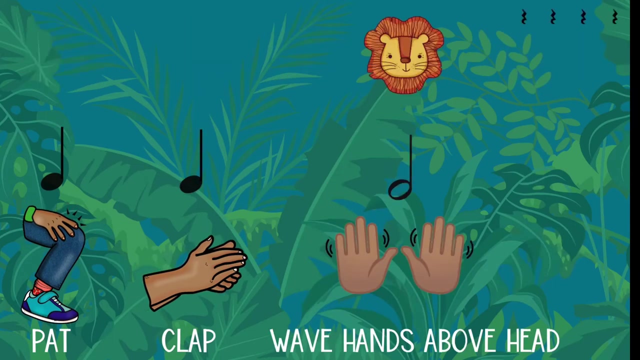 Everybody look right. Everywhere you look, I'm standing in spotlight. Not yet Let every creature know the broken sea. Let's see it in converting all the way. It's gonna be peace in the finest way. Oh, I just can't wait to be king. 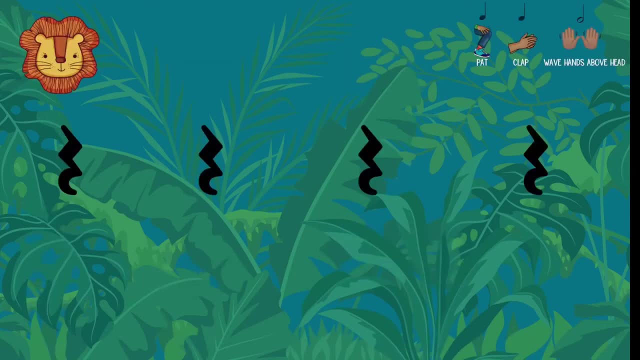 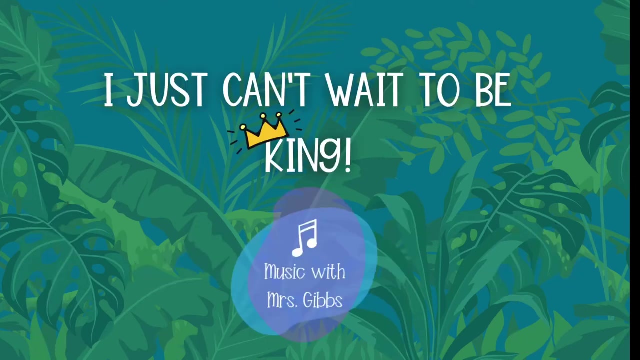 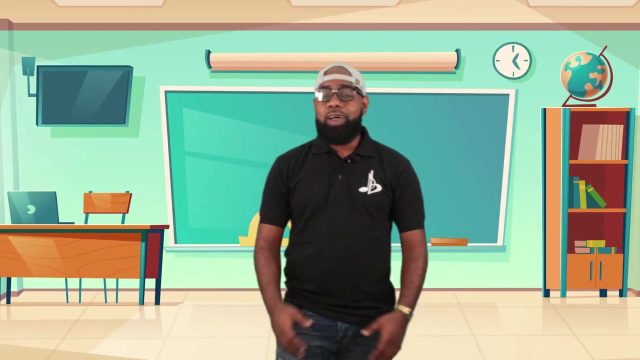 Oh, I just can't wait to be king. Oh, I just can't wait To be king. Whoa, that was awesome. I'm having so much fun. Rhythm is so awesome. I can feel it and I can say it. 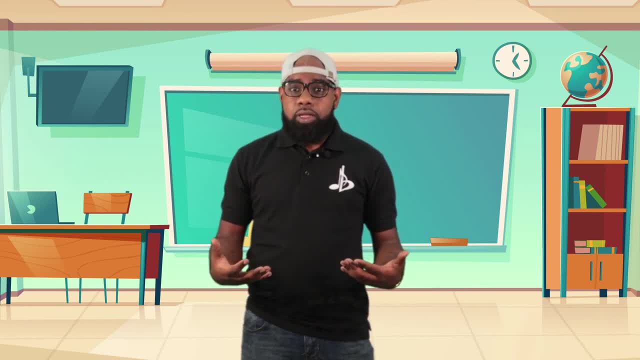 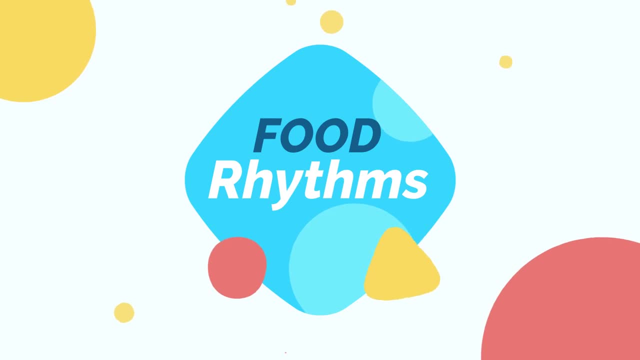 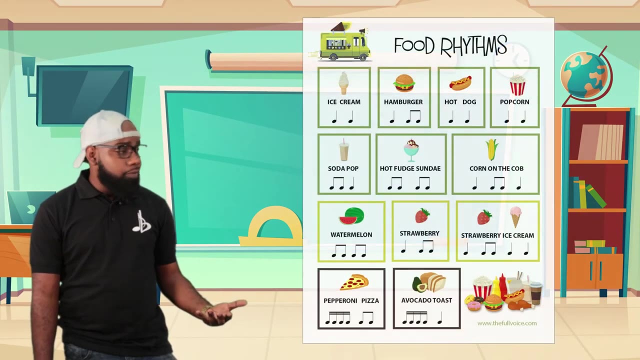 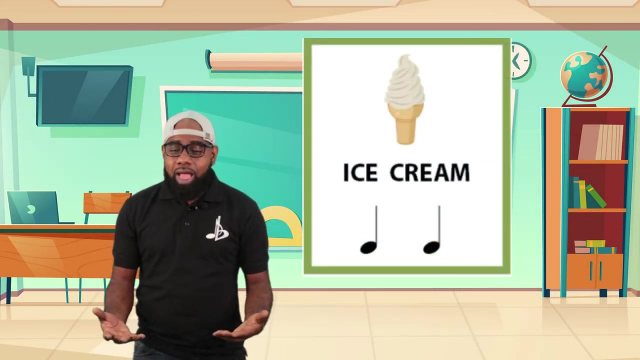 So let's apply rhythm to food. It's time for the food rhythms. Let's go. Can you see the food rhythms on the screen? Yep, I see them very clearly. Let's start with ice cream. Do you guys like ice cream? 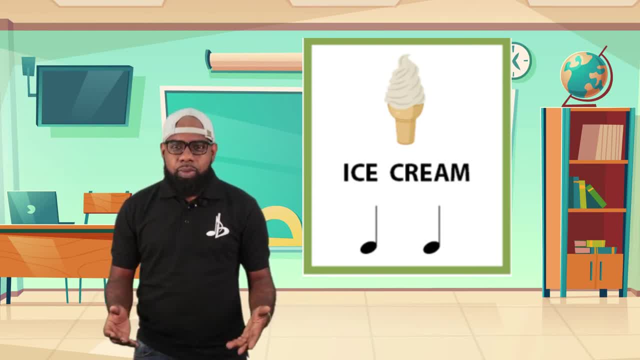 I love ice cream. So ice cream- What does that sound like? Let's check it out. Ice cream- Whoa, Can you do that with me? Let's go One more time. Ice cream, Excellent job, Excellent job. 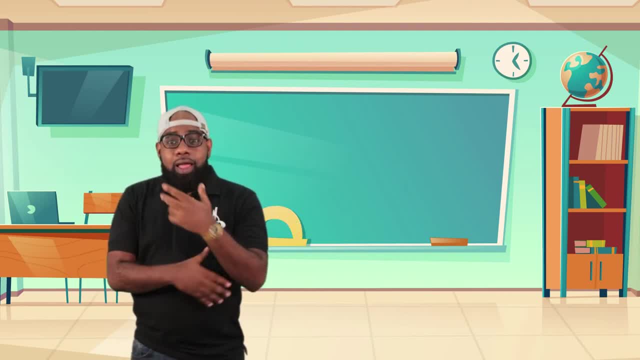 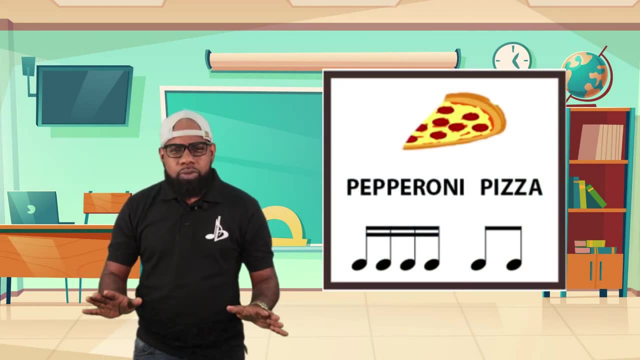 That was awesome. Let's try pepperoni pizza. That's long, Yep, So let's take our time. Pepperoni pizza: Whoa, I'm feeling hungry, guys. Okay, let's go, Let's go, Let's go. 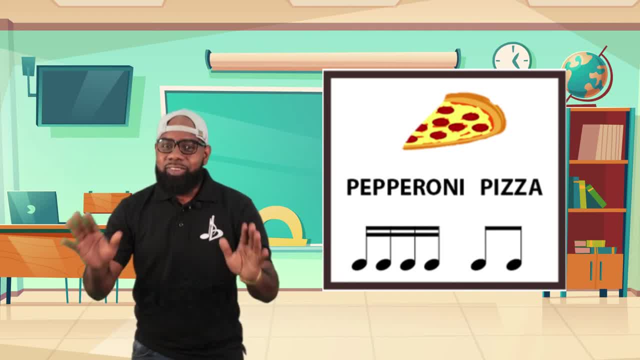 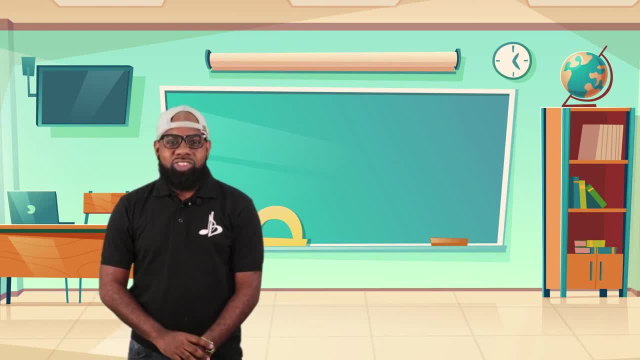 Pepperoni pizza: Whoa, Did you get that? Let's do it again. Pepperoni pizza. Excellent job, Excellent job. That's awesome. Let's try our next one. Like watermelon. Who doesn't like watermelon? I'm so hungry.